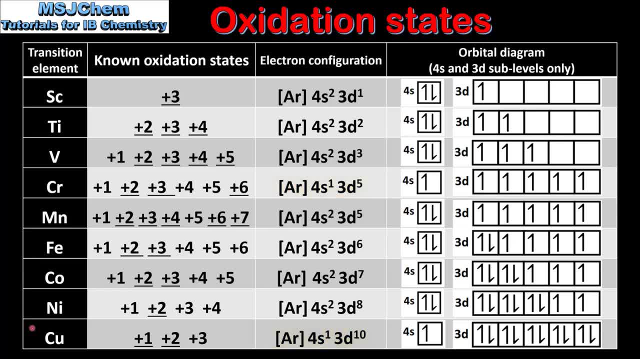 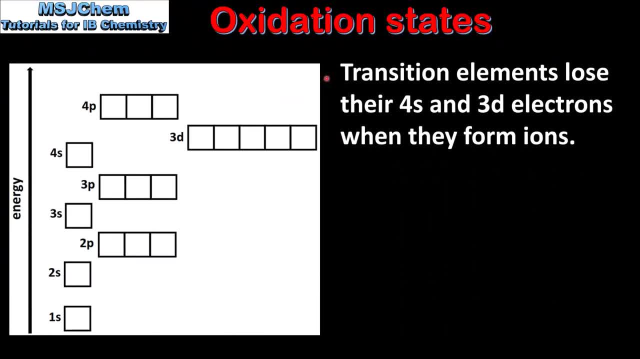 So next we look at why the transition elements have variable oxidation states. In the previous slide we saw that transition elements lose their 4s and 3d electrons when they form ions. On the left we have a diagram which shows the energies of the different sublevels. 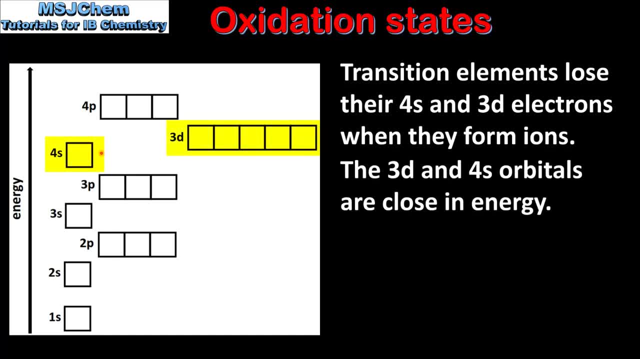 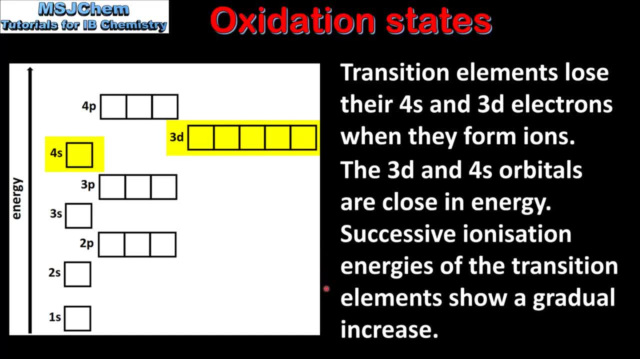 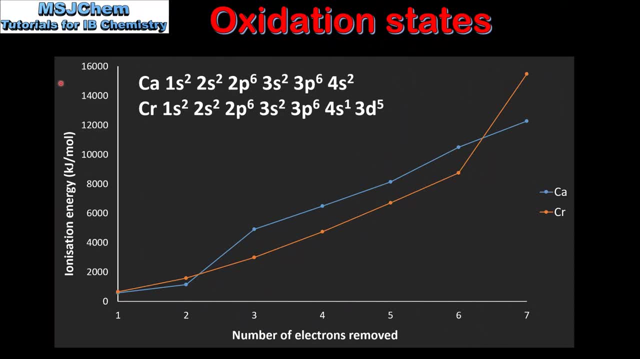 The successive ionization energies of the transition elements show a gradual increase. So this explains why the transition elements have variable oxidation states. Next we look at a graph which compares the successive ionization energies of two elements, That's calcium and chromium. Here we can see the electron configurations of both elements. 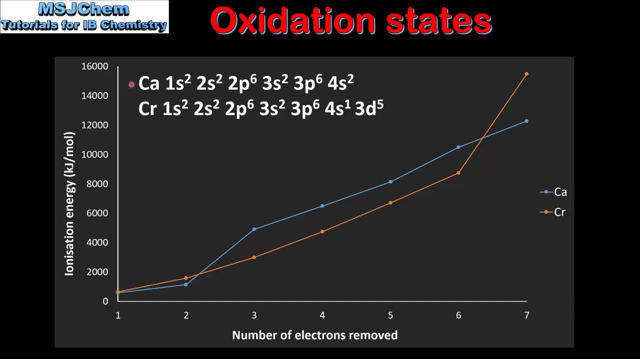 Calcium has one possible oxidation state, which is plus 2.. A transition element has variable oxidation states. So if we start with calcium, the first two electrons are removed from the 4s sublevel. We then see a large increase between the second and third ionization energies. 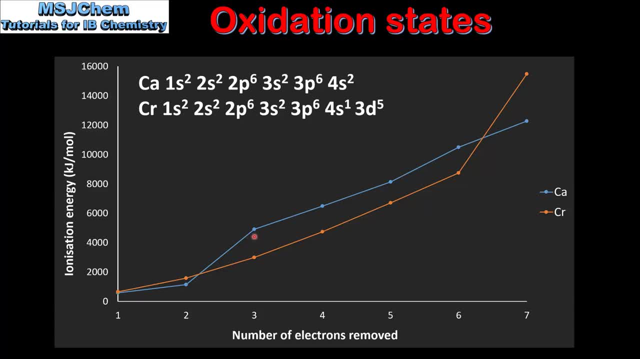 This large increase in energy is caused by the fact that the third electron is being removed from the 3p sublevel. The 3p sublevel is closer to the nucleus than the 4s sublevel. Therefore, electrons require more energy to be removed. So next, if we look at chromium, 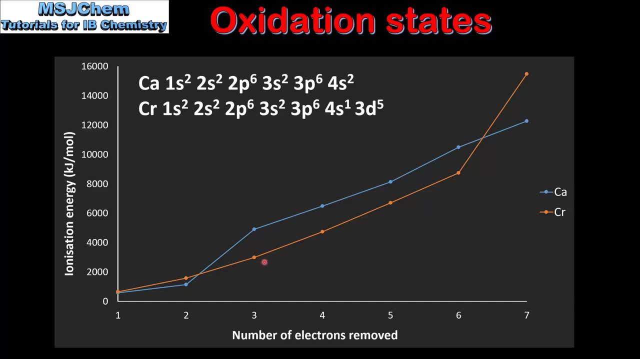 we can see there's a gradual increase in the successive ionization energies. The first electron is removed from the 4s sublevel and the next five electrons are removed from the 3d sublevel. The large increase in ionization energy occurs between: 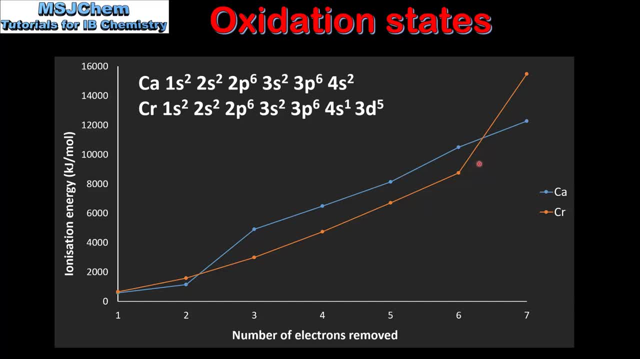 the sixth and seventh ionization energies. This is because the seventh electron is removed from a 3p- 3p sublevel. Just like in calcium, the 3p sublevel is closer to the nucleus. therefore, electrons in this sublevel require more energy to remove. So this explains why chromium, like all transition,